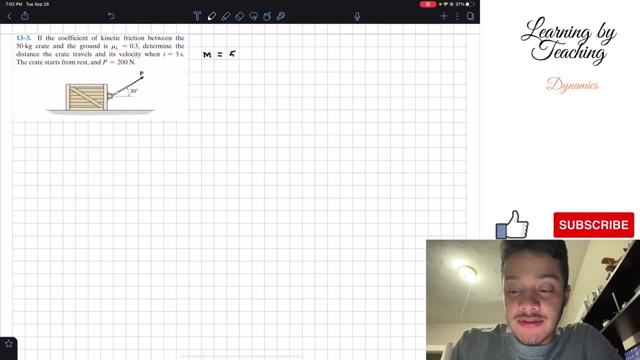 my givens first. So first we're given that our mass is equal to 50 kilograms, Then we're given that the kinetic friction is equal to 0.3.. We're also given that the time that we want to find this distance and velocity is equal to 3 seconds And our force p is equal to 200. 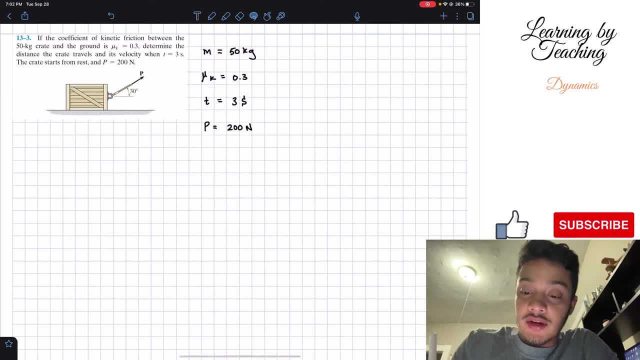 nits. Okay, So, these here are our givens, and we're asked to find the distance d or s, and our velocity. Okay, So, in order to start this problem, since we need to calculate the sum of material forces, the first thing, 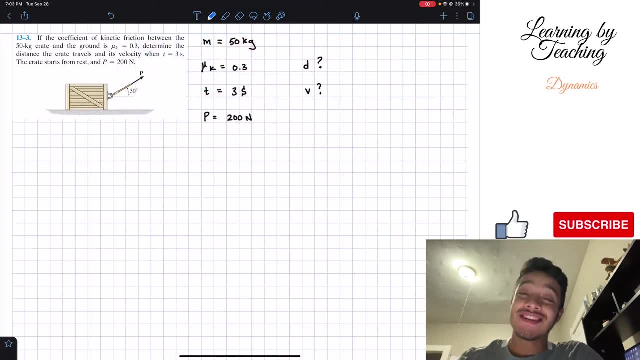 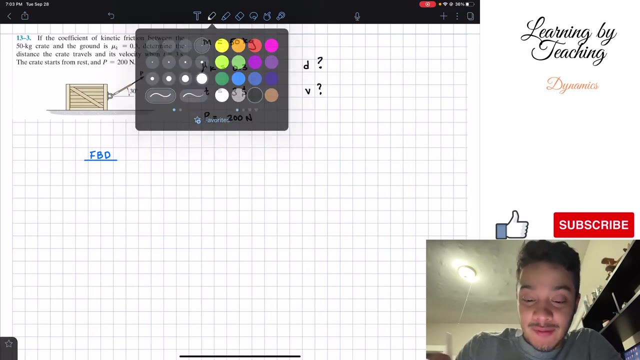 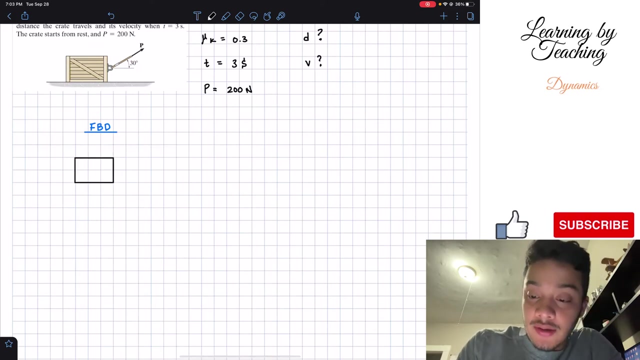 that we need to do- and going back to our statics videos- is sum of material forces. Okay, So I'm sorry, free body diagram. So we're going to go and do a free body diagram for this problem. So we got our free body diagram and the crate looks something like this. So we got our rectangular 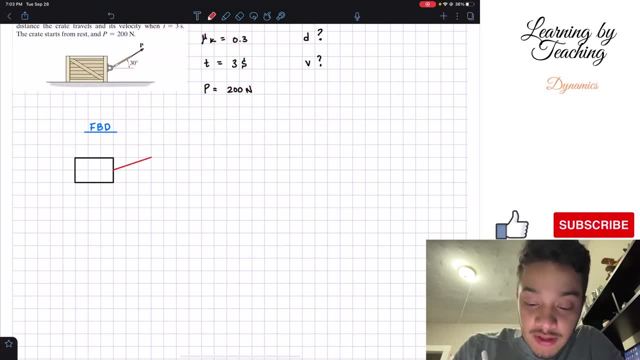 shape. We've got a force p pulling at a 30 degree angle. That looks something like this: We know this piece equal to 200 newtons, And let's state that the angle is 30 degrees. Okay, That's good for that. We have the friction that is occurring. 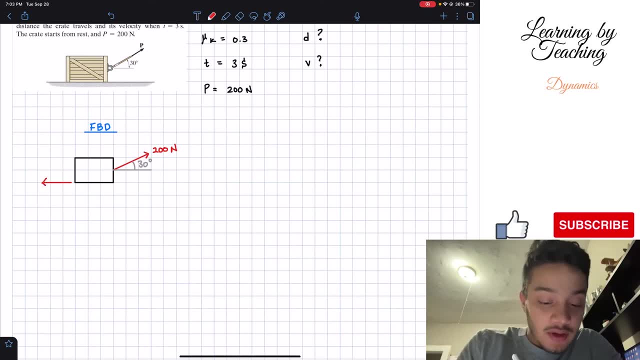 between the crate and the floor- that we're going to call it f- of friction. We have the weight of this crate going down- that we're going to call it w- and we have a normal force Opposite to the weight. Okay, so this is how our free body diagram looks like. 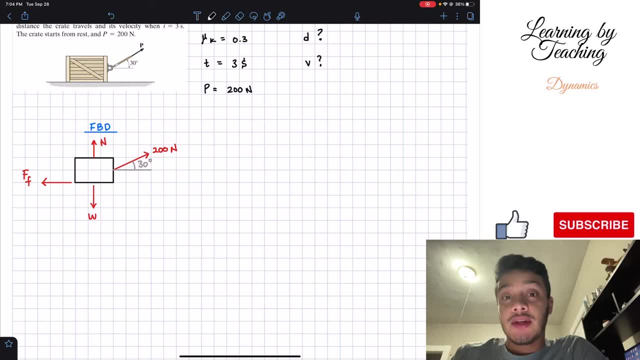 And we're going to start With our somatario forces in the y direction. and the reason why we're starting with the somatario forces in the y direction Is that we're moving horizontally Through the right, but In the vertical position we're neither moving up or down. 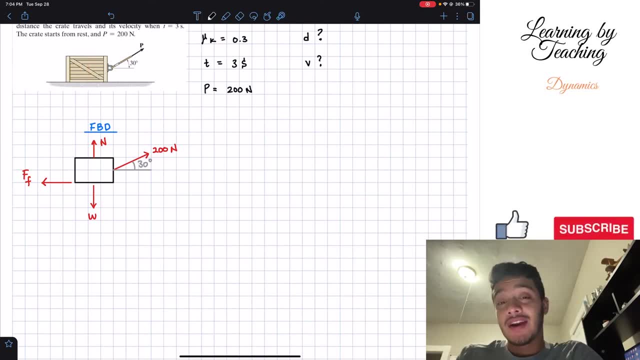 Therefore, our acceleration is equal to zero and our somatario forces should be equal to zero. So we got, somatario forces In the y direction should be equal to zero. Okay, we're going to assume that going up is positive and Since we know that, then what are the forces that I have in the y direction? Well, I have. 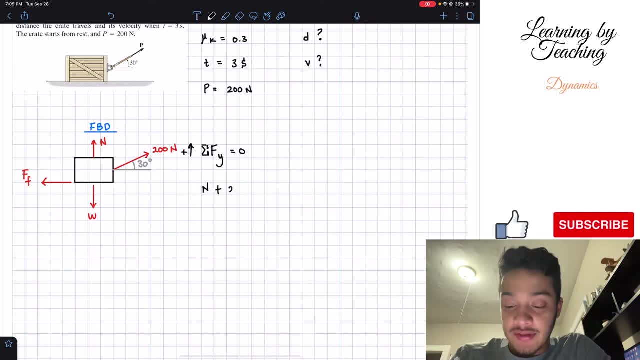 positive normal force. Then I have positive The y component of this: 200 newtons is going to be 200 multiplied by the sine of my angle, sine of 30 degrees. And lastly, I will have minus w, Okay, And all this should be equal to zero. 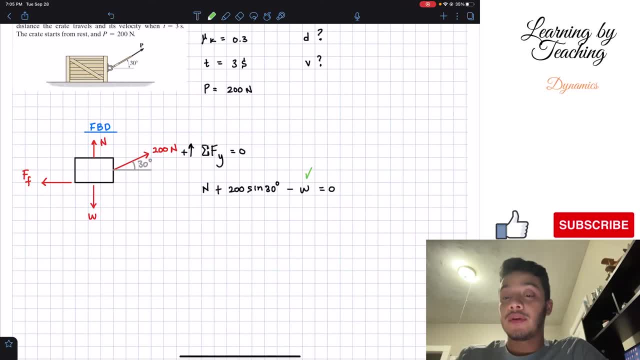 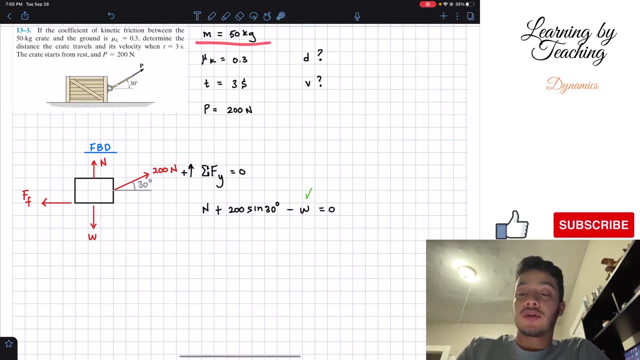 So, taking into account, we do know our w and the reason for that Is that we know how much is our mass for this crate, which is equal to our 50 kilograms That is given in here. So if we solve for n, we're going to have: 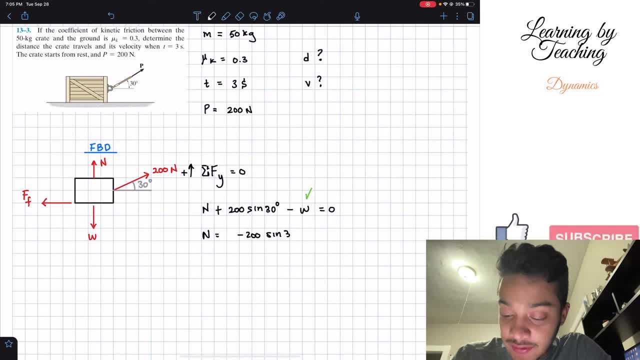 negative 200, multiplied by my sine of 30 degrees plus W. well, w is going to be my mass, Multiplied by my acceleration in the y direction, which is 9.81, our gravitational acceleration. And I think that's it All right. So we're going to plug this into our calculator and let's see how much we get. 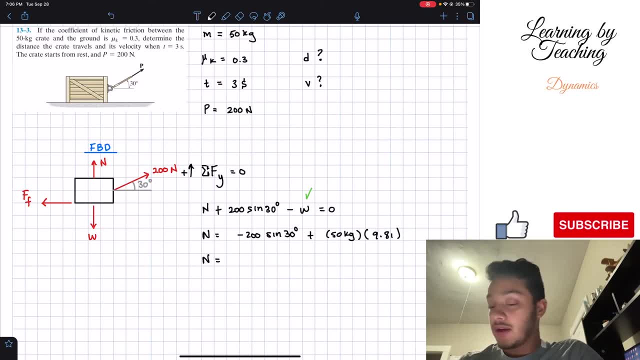 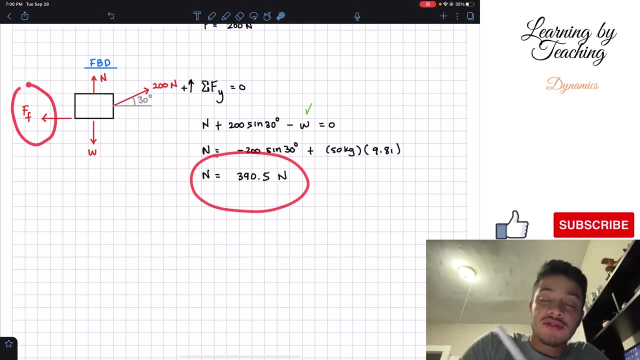 So if we plug this into our calculator, we should get a total of 390.5 Newtons. okay, So we found on a normal force, And the reason why we're trying to find this normal force is because this frictional force is dependent of our normal force. 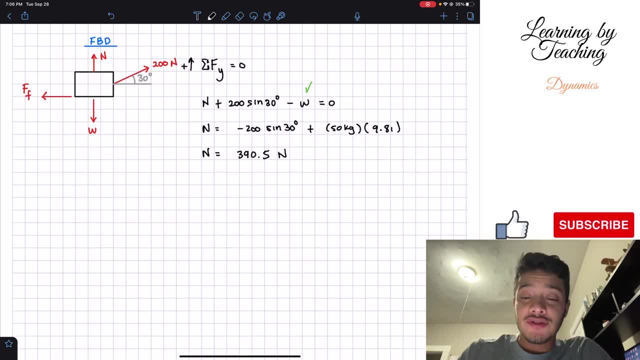 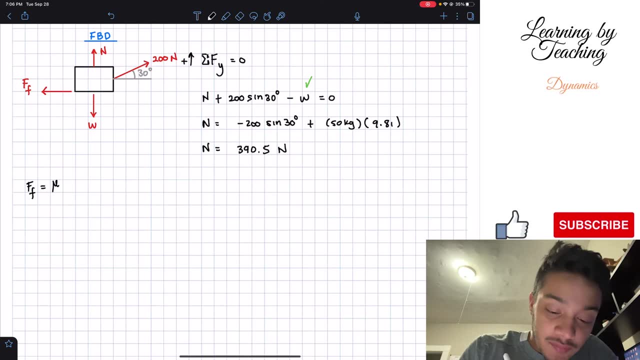 now, if you remember about statics, our frictional force is fun. and it's fun because the frictional force is equal to mu Multiplied by n, so it's f? u? n fun. now, If we calculate and we plug our numbers, mu is giving us 0.3. 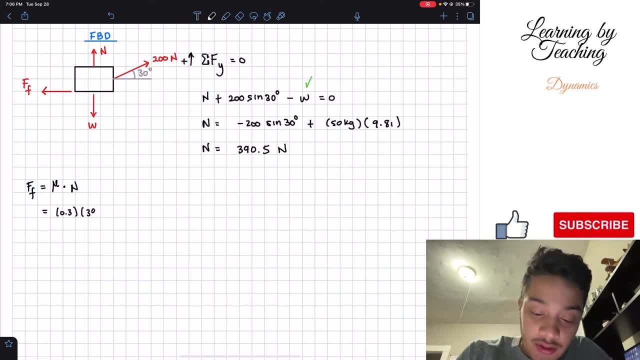 by the problem And our normal force is our 390.5 newtons that we just calculated, And if we plug this into our calculator, we will get a total of 117.15 newtons for our frictional force. Okay, Now that we know our frictional force, we can start applying our sum of the real forces. 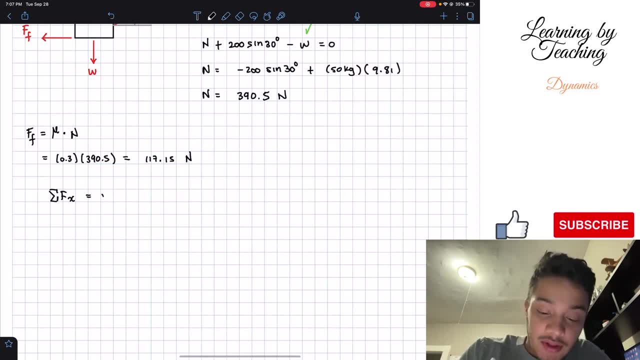 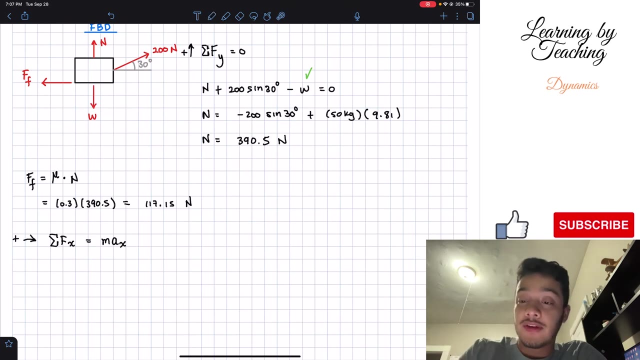 In the x direction, but in this case, these are not going to be equal to zero, They're going to be equal to mass times acceleration in the x direction. Okay, we're going to assume that going to the right is positive And therefore, what do we have? well, we can start with our frictional force. is going to the left meaning that is negative? 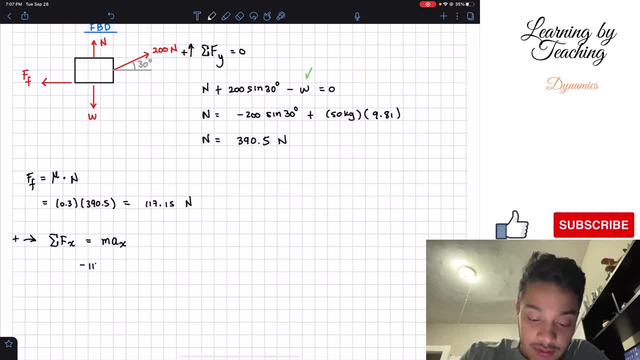 So we got negative frictional force 117.15. Then we have positive, this x component of the 200 newton, so we got plus 200 multiplied by my cosine of 30 degrees, Gotta be equal to my mass times acceleration in the x direction. 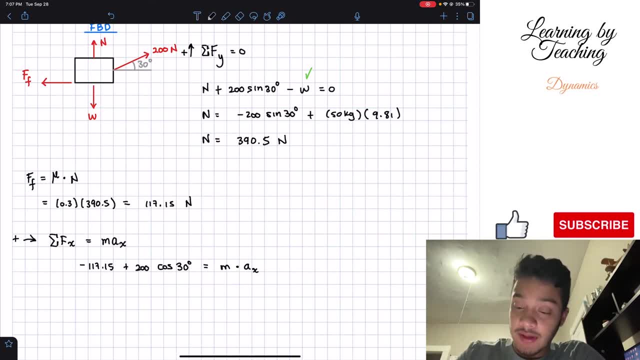 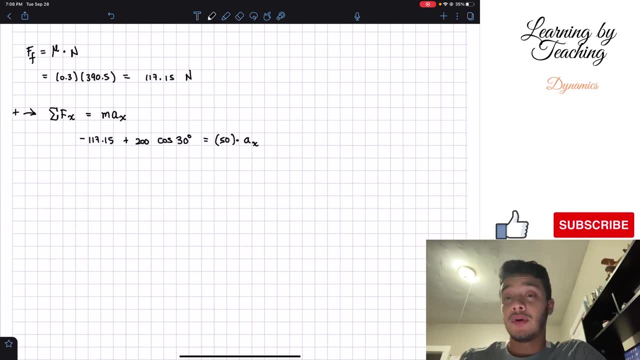 But we also know how much this mass is, which is 50 kilograms. so we can replace this m with 50 and We'll have an equation with only one unknown. so we can solve for my acceleration in the x-direction, Which will be one: 17 positive point, 15 plus, I'm sorry, minus, in this case 200 cosine. 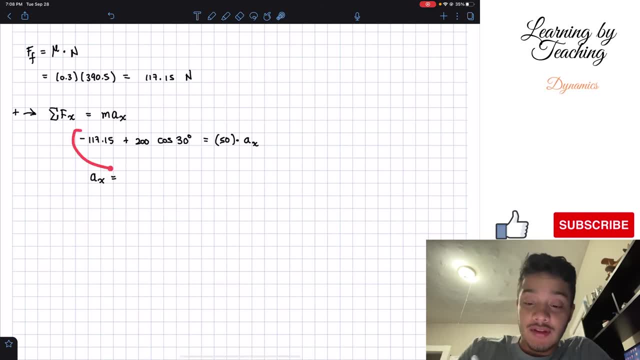 I'm sorry, I've been. I got confused. We're not moving these guys over here, We're moving this 50. So our acceleration in the x-direction is going to be one 17 negative point 15 plus 200 cosine of 30 degrees. 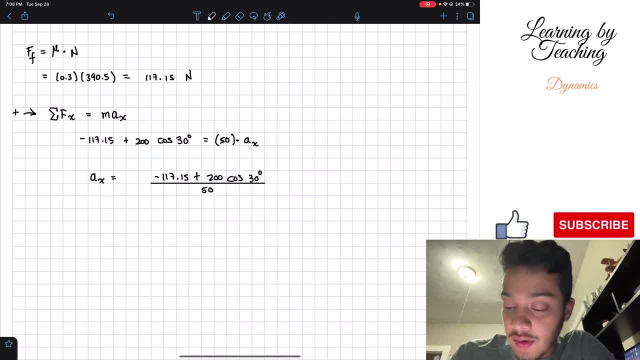 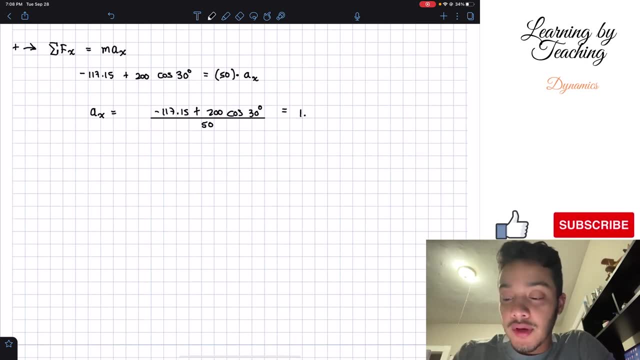 all divided by 50. Okay, and if we plug this into our calculator, let's see how much this is. This will give me a total of one point, one, two, And this is in meters per second squared. So now that we reach our acceleration, But we're being asked to find velocity. 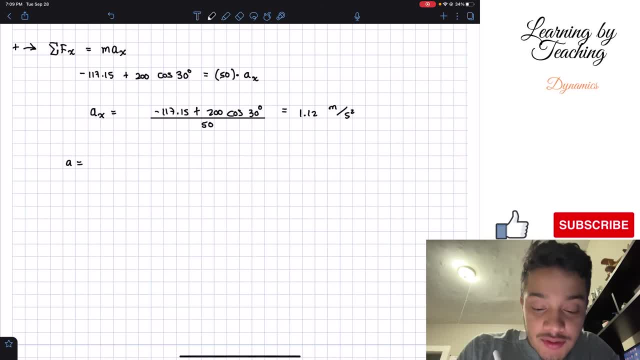 Therefore, what we need to know is that our acceleration is equal to our change in velocity divided by our change in time. If we solve for our change in velocity, we will realize that this is equal to our acceleration times, our change in time. okay, Later on, when we find velocity, we will also need the relationship that our position, our velocity, 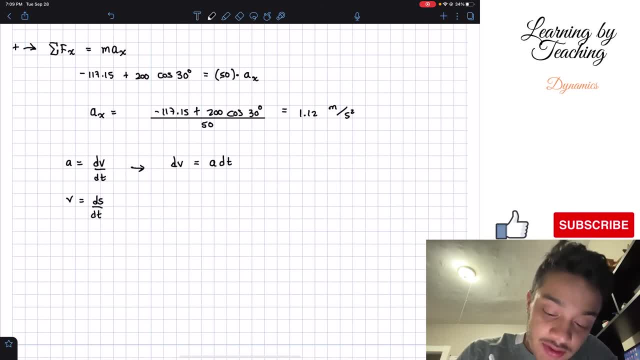 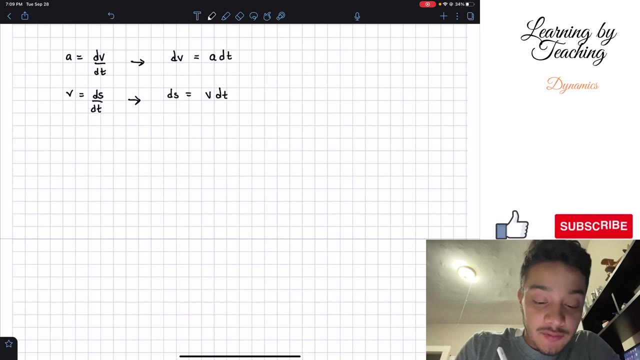 Is equal to our change in position divided by our change in time. And if we solve for our change in position, we will have velocity times, the change in time. okay, So we're going to utilize These two relationships in order to find our velocity and position, and starting from our velocity, 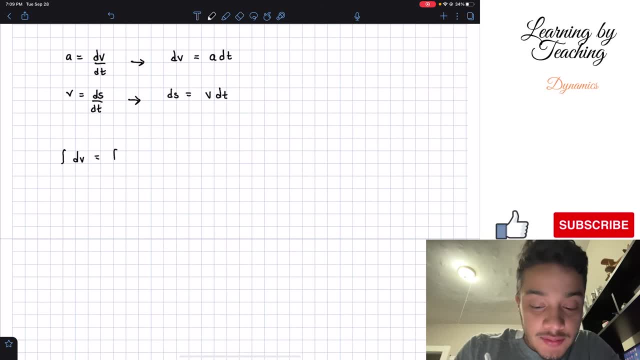 We're going to have, the integral of our change in velocity has to be equal to the integral of our acceleration times, the change in time. Okay, now our velocity starts at zero, because this starts our rest And our final velocity. we're just going to call the v. 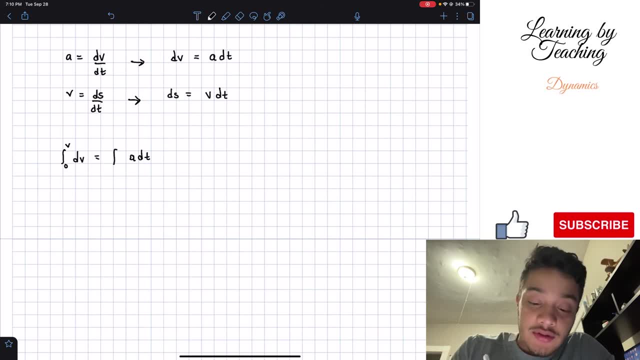 for our acceleration. we're going to start uh For our time. since we're doing derivative with respect to the change in time, We're going to start at zero and we're going to end up our t final t. Okay, we can replace our acceleration. 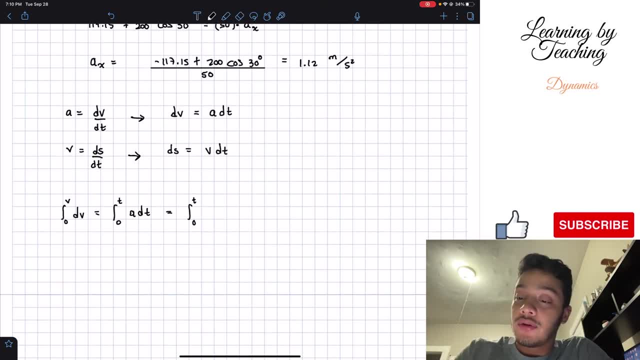 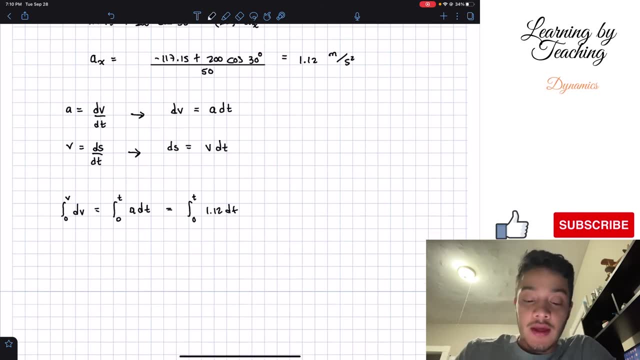 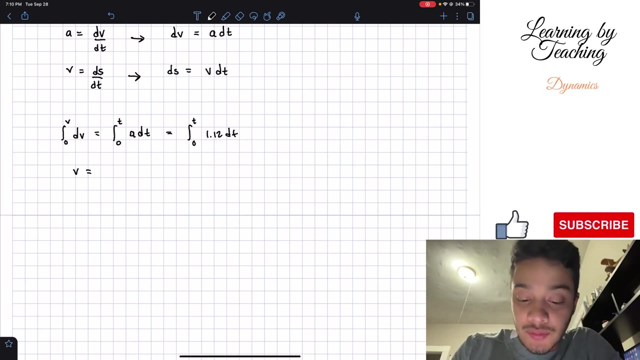 for The acceleration that we found to be 1.12. So we got 1.12 dt If we solve the integral on the left side, we have, But that v has to be equal to 1.12 times t. Okay, and now we found our velocity equation. 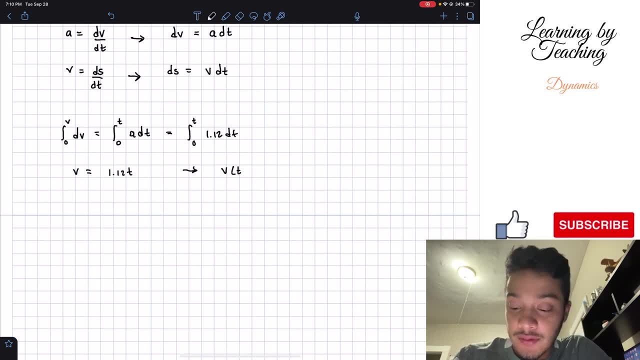 If we want to find our velocity when time is equal to 3, so velocity when times equal to 3- We're just going to plug 3 into our equation And we'll have 1.12 times 3, And if we plug this into our calculator, 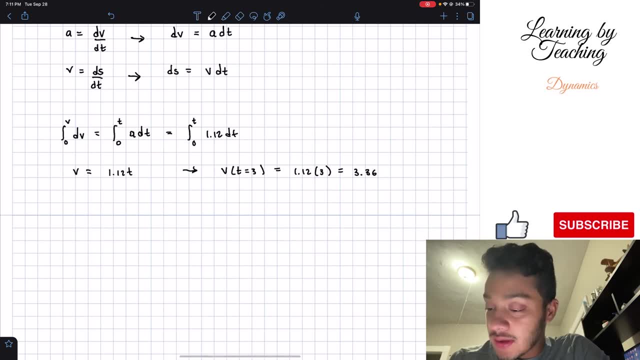 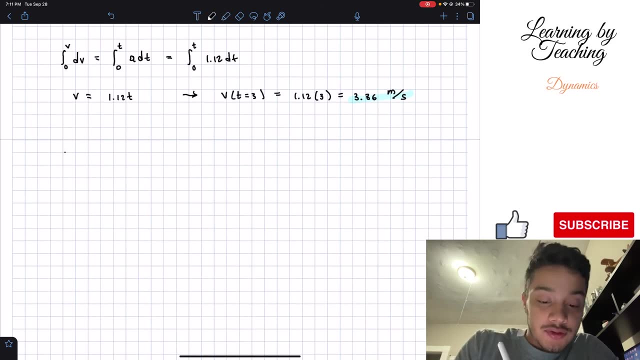 We'll get a total of 3.36 meters per second. Okay, so this is our first answer. Then later we're going to apply a same concept: that our change in position has to be equal to our velocity times change in time. Our position starts at zero. 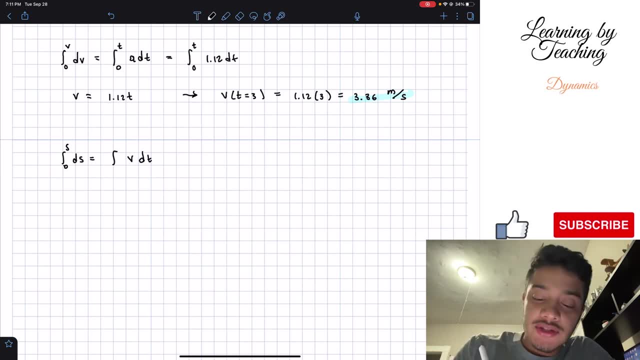 final position. We're going to call the s for final position and then our time starts at zero. And our final time? we're just going to call it. We can replace our velocity For the velocity equation we just found in terms of time. Therefore, we're going to have: